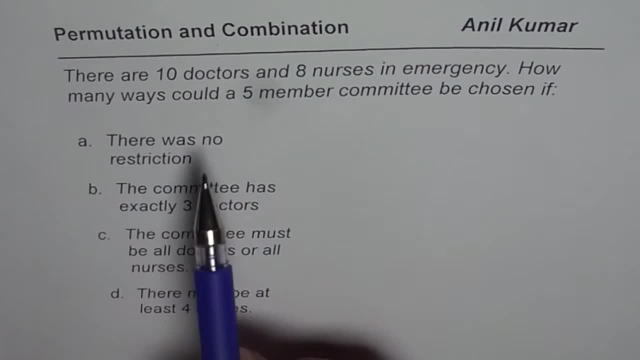 The very first one that we are selecting a committee of 5 members From 10 doctors and 8 nurses, And there are no restrictions. So basically, what we have here is: total number of persons are 10 plus 8, 18.. So N is 18.. So what we have here is: 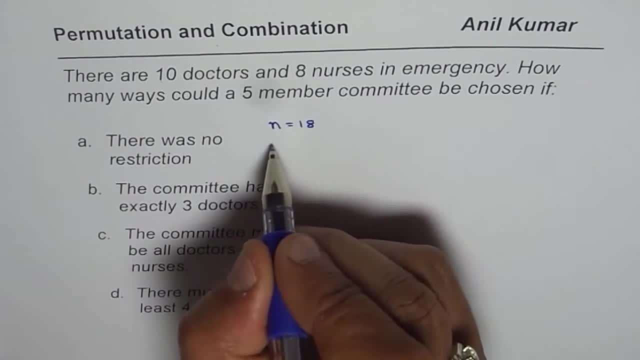 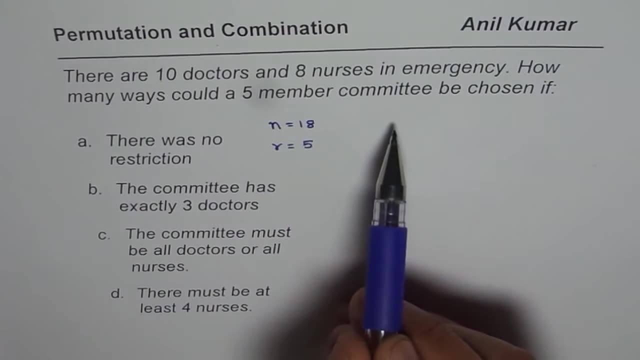 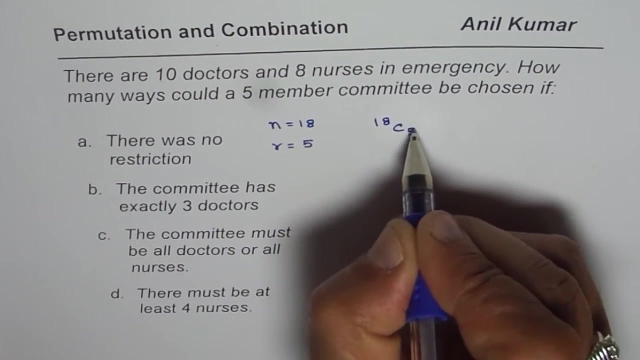 N equals to 18. And we need to select 5.. So R is 5. And since it is a committee, all have the same status. Correct, Correct, And therefore the solution is 18C5.. So that becomes the number of ways in which this committee can. 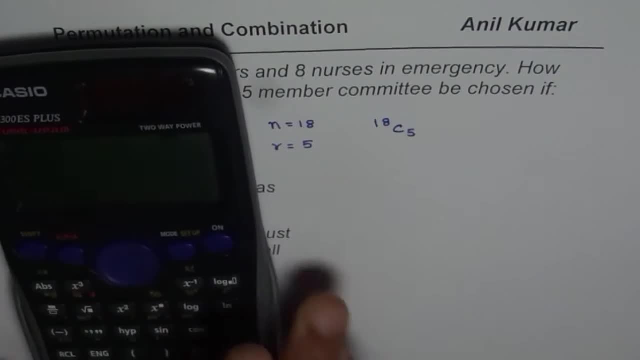 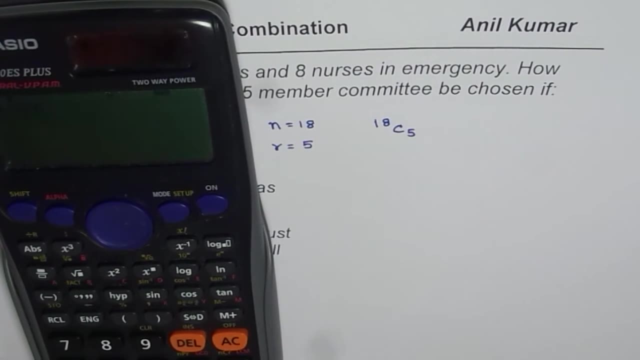 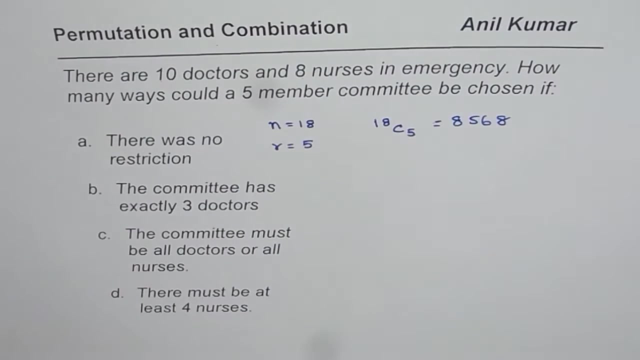 be selected, So you can always use your calculator, find the answer. It is 18 and the NCR formula right 5 equals 2.. So we get the result as 8568,. right Now Part B. Part B. 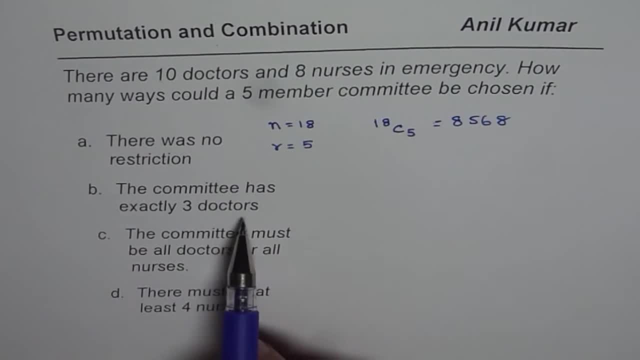 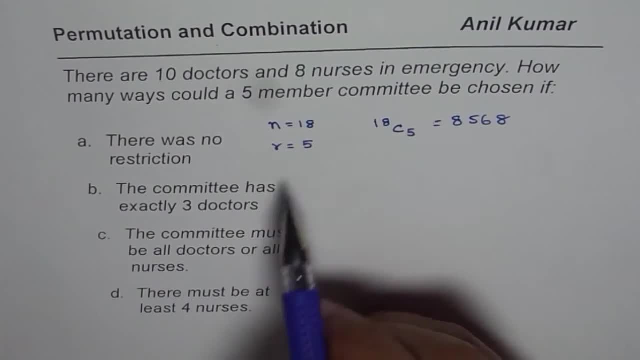 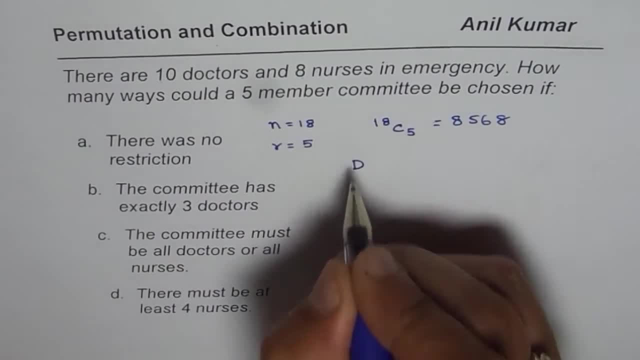 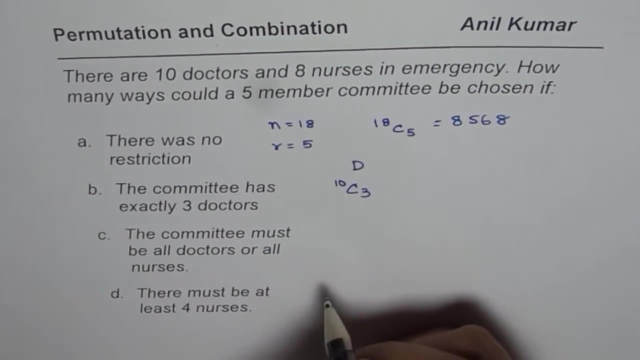 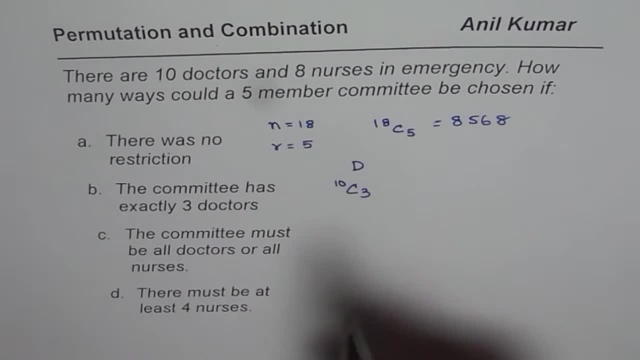 rest of nurses: right. exactly 3 doctors, so 2 out of 8.. So from 8, we have 2, right. So that is the number of combinations. Now, in this particular case, since this is followed by that and right, that means it gets multiplied. So that becomes the answer for Part B. So 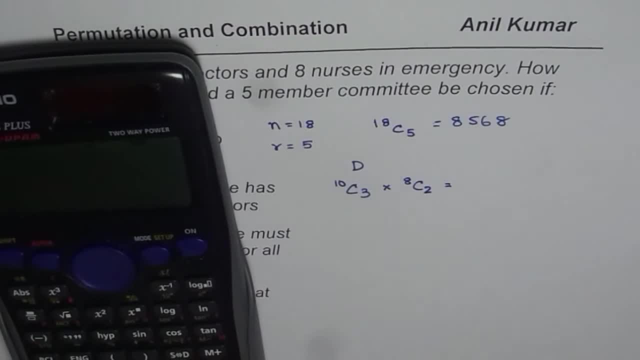 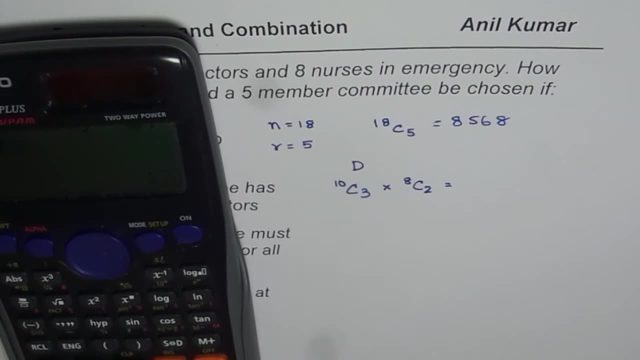 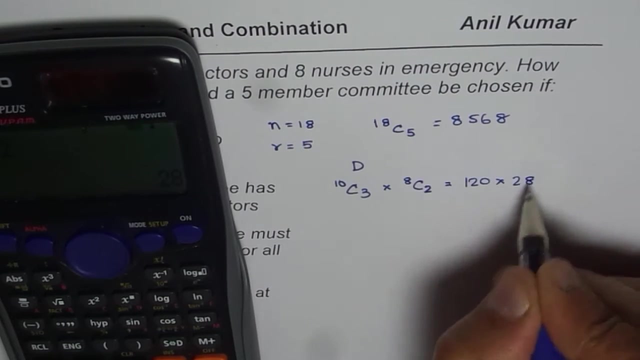 let's calculate this answer: It is 10 C. R is 3, equals to 120 times 8, C2.. Okay, Which is 28,, right? So when you multiply this, you get 28 times 120 as equals to 3360, right? 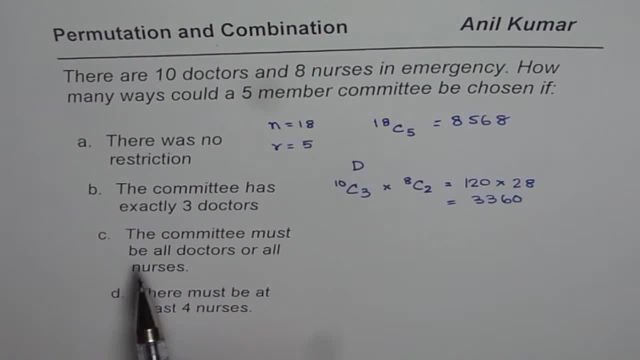 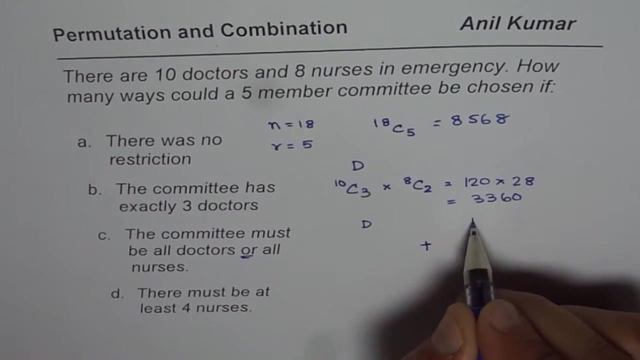 So these are the different number of ways. Part C is the committee must be all doctors, or or means plus right, all nurses. So we have now the operator, or that means plus all doctors or all nurses. So that is what it is. 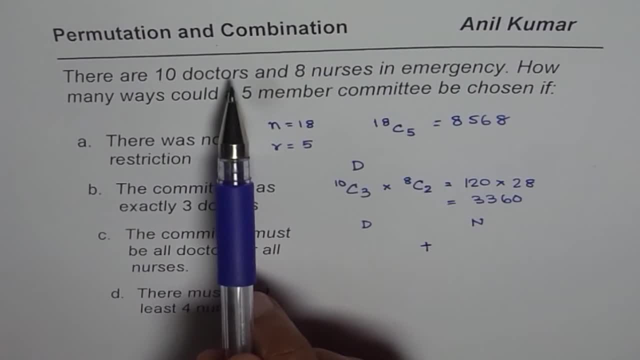 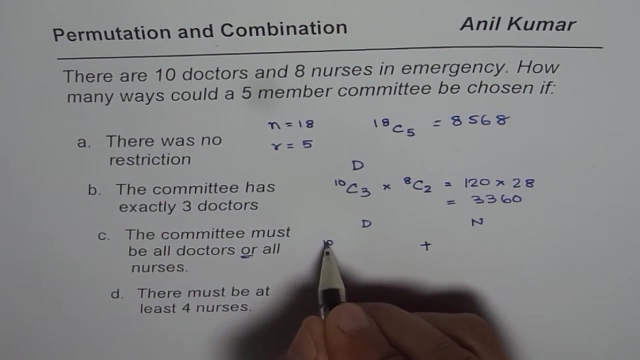 Now there are 10 doctors, so we are selecting 5 members, right? So that means we have to select 5, all doctors means 5 out of 10, and that gives us the combination 10C5.. Now if 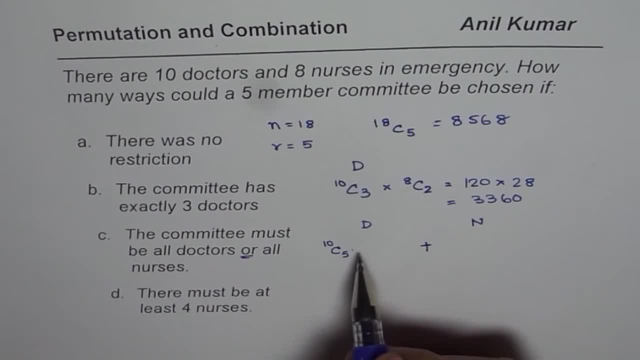 you do this selection, then as far as the nurses are concerned, none of them is selected from 8. So you may write 8C0, which you know is correct, Okay, Okay. So 8C0 is 1, right, So 1 times anything is that number itself. Now, if you select all, 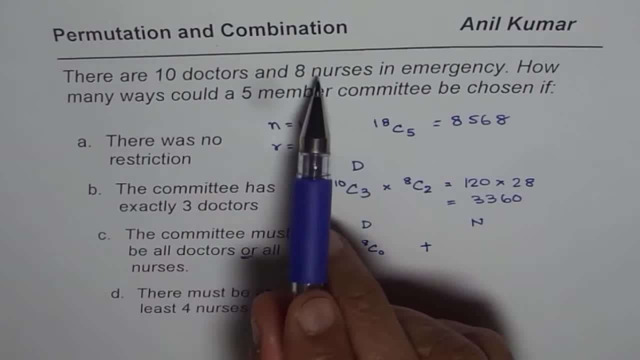 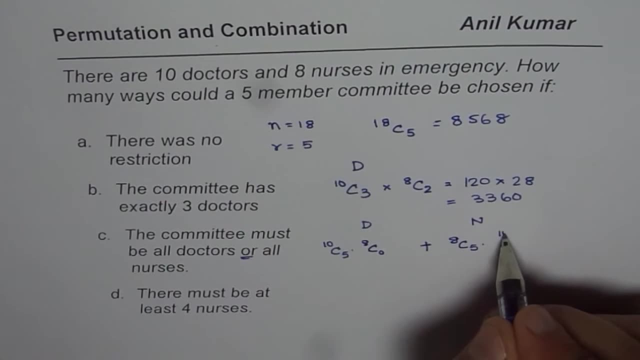 nurses. that means you are selecting 5 out of 8, and therefore it is 8C5 times. no doctors are selected this time, So 10C0.. And you can use the calculator to find this answer. Let's calculate. 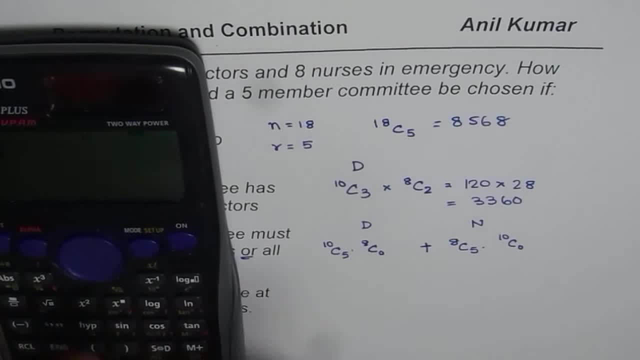 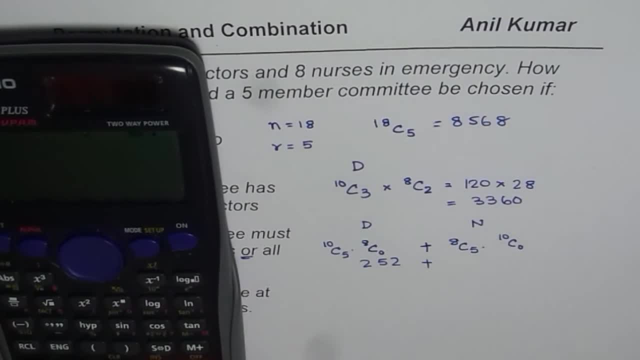 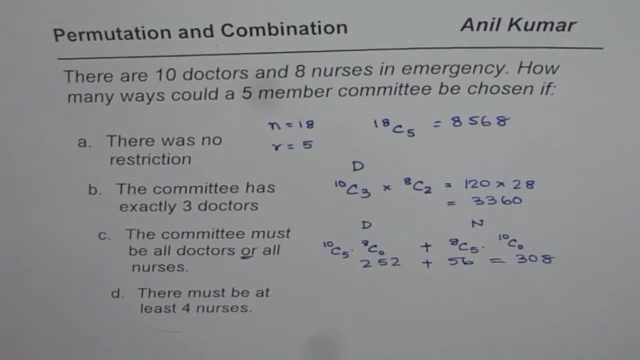 8C5.. So 8C5 equals to 56. And when you add them up- let me add 252 to 256, we get 308 as our answer right. So let's look into Part D, which is there must be. there must be a. 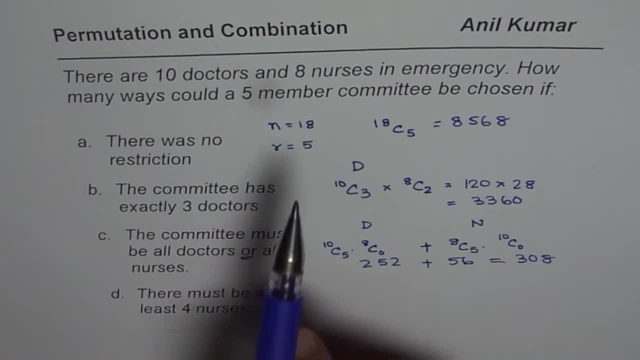 committee at least 4 nurses. Now we are having a committee of 5 members. at least 4 nurses means you could have 4 nurses or you could have 5 nurses. So when we say or, that means we need to add it up, correct. So that is what it is. Now, if you select. 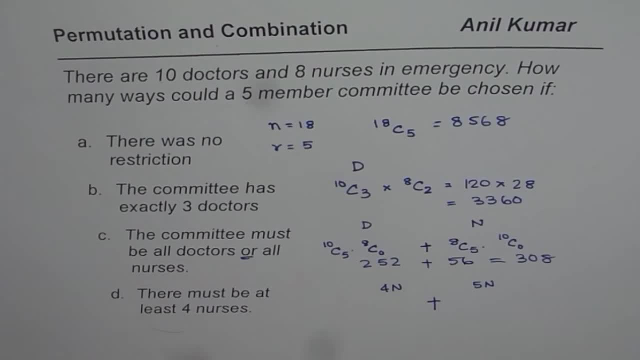 4 nurses. these are being selected from 8 nurses, right? So we can say I mean 8C4, right, Okay? Okay, So that is selecting 4 nurses. Since we need a committee of 5 members, 1 doctor is selected. 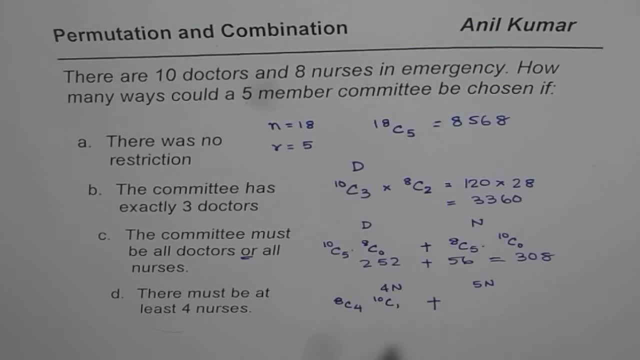 right, So it is out of 10,. 1 is selected Plus 5 nurses means out of 8, we select 5, and then the number of doctors will then be 0, right, So it would be 10C0.. So we can calculate. 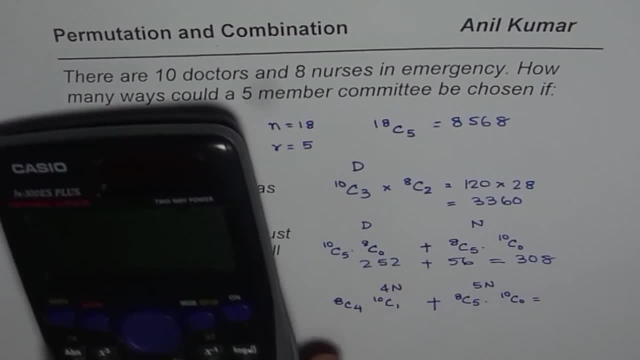 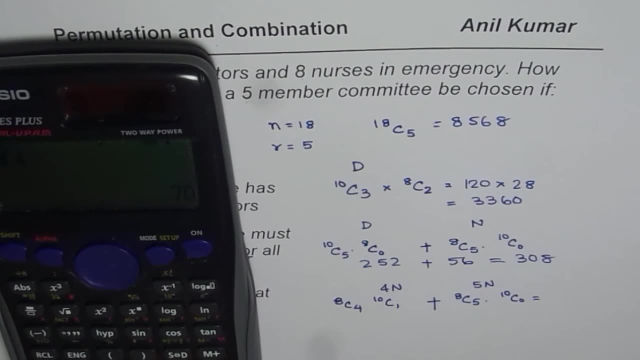 this and find the answer correct. So it gives us 8C5.. Okay, Okay, So 10C4, which is equal to 70, 10C1,, you know, is 1.. So that is 70 plus 8C5, and that. 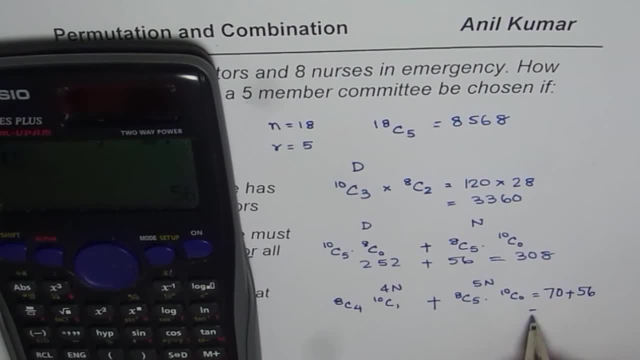 is 56,, 56. And that gives you the value. as sorry, we didn't know, multiply by 10C1, but 10C1.. That should be multiplied by 10C1.. So 10C1, which is 10, I should have multiplied this. 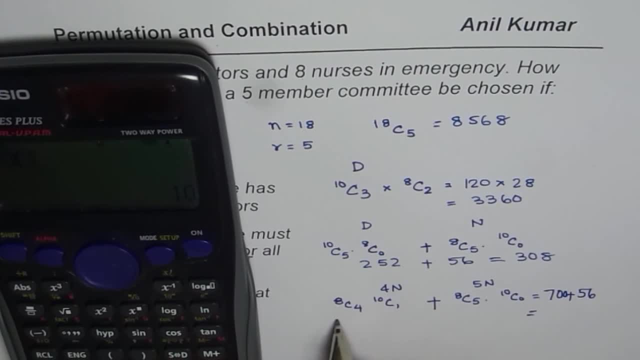 by 10.. So that is 700,, right 700.. So it is 70 times 10 plus 8C1 is 56 times 10C0 is 1.. So we get 756 as the result. Okay. 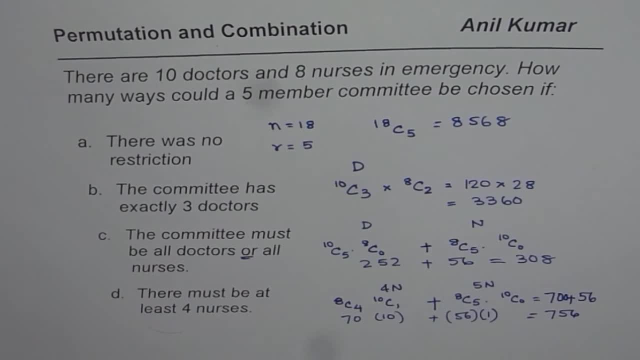 Okay, So how you can solve such questions. Now, it is very important to understand that when you are selecting different kinds of committees, you need to see when to add and when to multiply. So when there are options with or, then you are adding right, And whenever there is an